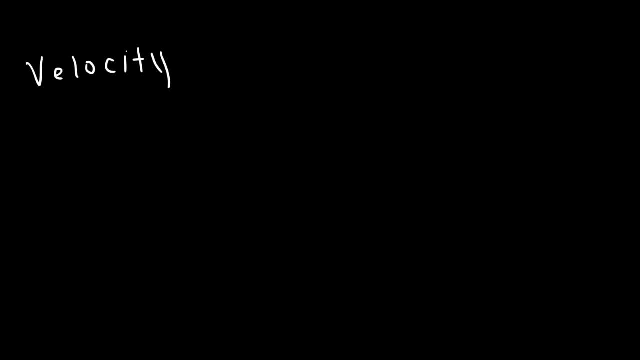 Velocity tells you how fast an object's position is changing with respect to time. So basically, velocity is the displacement, which is the change in position over time. So V is equal to the displacement, is the final position minus the initial position divided by the elapsed time. 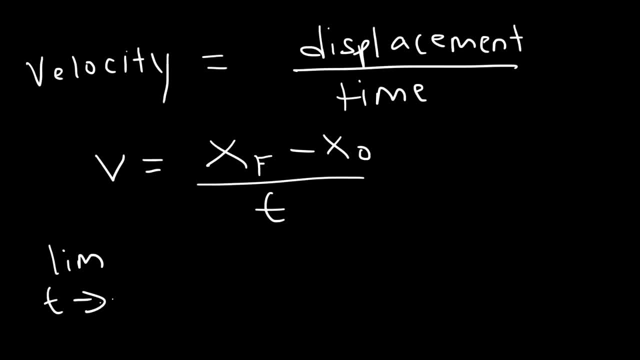 Now, as t approaches zero, this expression is, or becomes, rather the instantaneous velocity. The previous equation represents the average velocity. So if you want to find the average velocity, simply use this equation. It's the position, I mean, it's the change in position over time, or displacement over time. 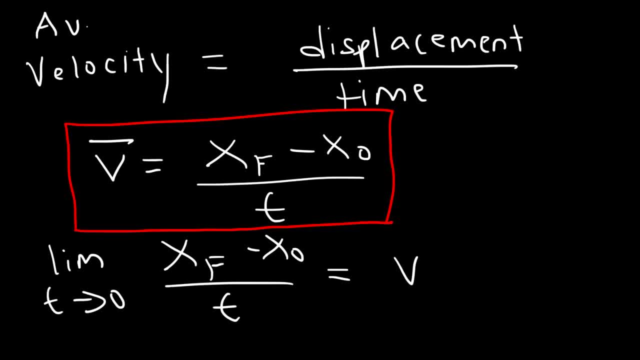 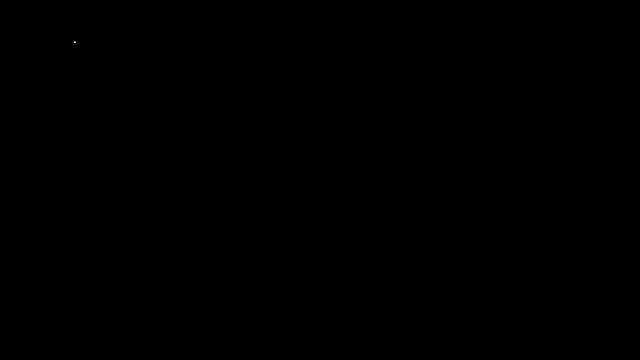 So that will give you the average velocity, Whereas the instantaneous velocity. you can use the same formula, but when t becomes very, very small, it will give you the instantaneous velocity. Now let's say, if you have a car that's moving at 30 miles per hour, 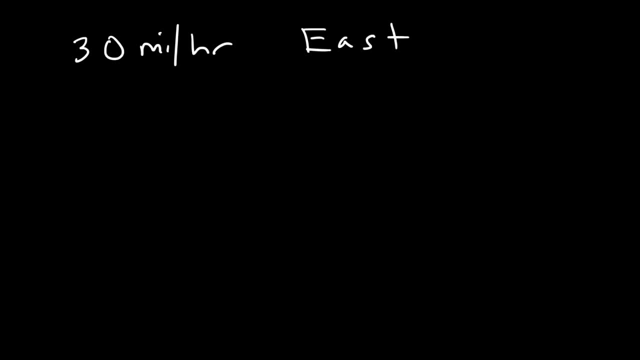 traveling east. So this expression, the magnitude and the direction, that represents the velocity of the vehicle. So every hour the car travels a distance of 30 miles. So in 2 hours it's going to travel 60 miles, 3 hours 90 miles. 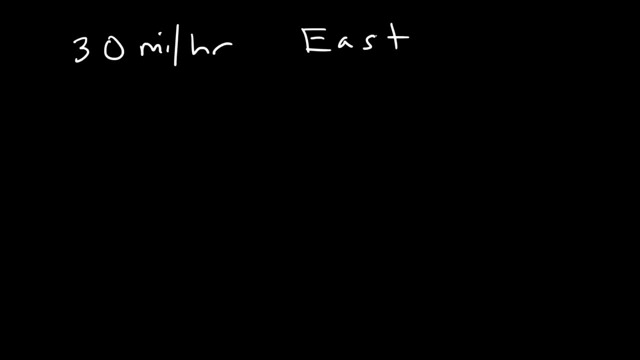 So speed tells you how fast the distance is changing. Velocity tells you how fast the displacement is changing. So let's say if a car, or let's say if an object is moving at a speed of 8 meters per second. 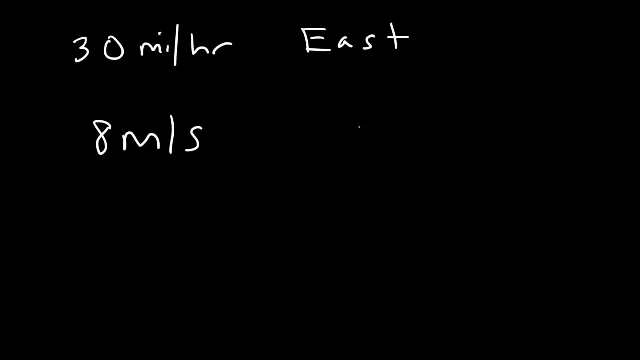 Every second the distance is changing by 8 meters. So after 1 second the distance traveled is 8 meters. 2 seconds, 60 meters. 3 seconds, 24 meters. So that's the main concept between speed and velocity. 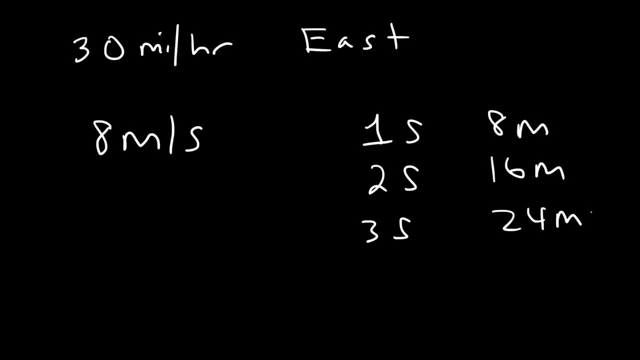 It tells you how fast the distance, or the displacement, is changing Every second. So if a car is moving at a speed of 15 meters per second, every second the distance is changing by 15 meters. So to sum up what we just considered: 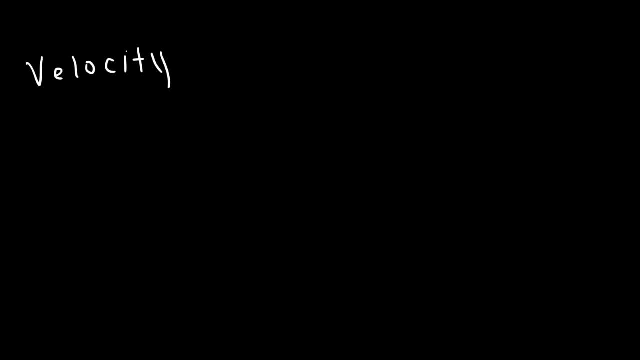 Velocity tells you how fast an object's position is changing with respect to time. So basically, velocity is the displacement, which is the change in position over time. So V is equal to the displacement, is the final position minus the initial position divided by the elapsed time. 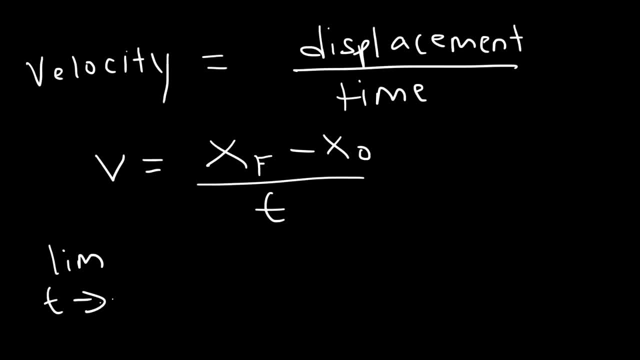 Now, as t approaches zero, this expression is, or becomes, rather the instantaneous velocity. The previous equation represents the average velocity. So if you want to find the average velocity, simply use this equation. It's the position, I mean, it's the change in position over time, or displacement over time. 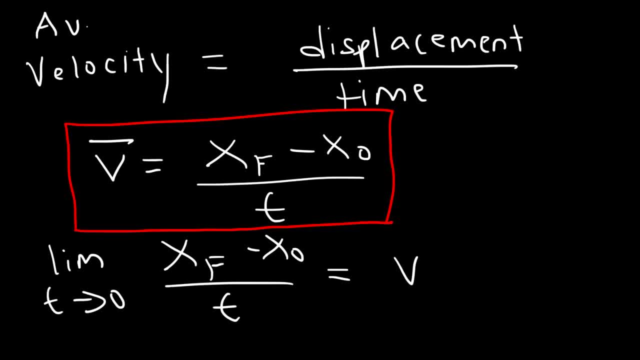 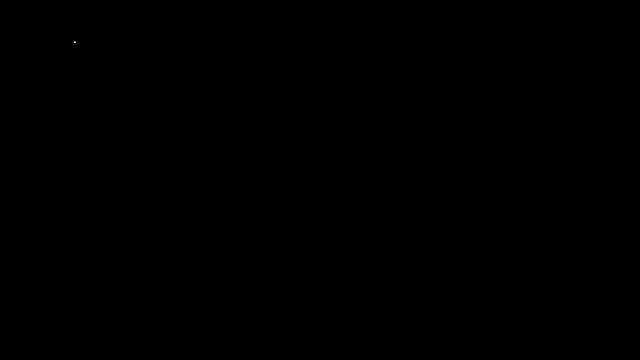 So that will give you the average velocity, Whereas the instantaneous velocity. you can use the same formula, but when t becomes very, very small, it will give you the instantaneous velocity. Now let's say, if you have a car that's moving at 30 miles per hour, 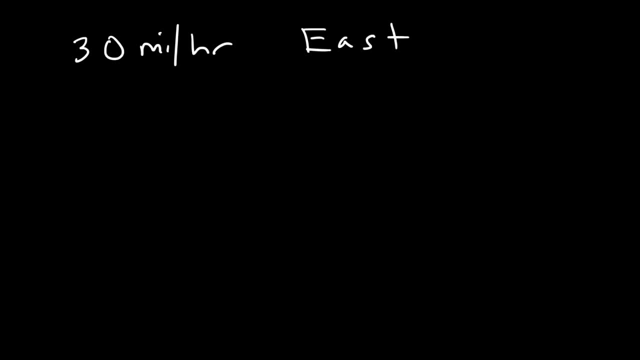 traveling east. So this expression, the magnitude and the direction, that represents the velocity of the vehicle. So every hour the car travels a distance of 30 miles. So in 2 hours it's going to travel 60 miles, 3 hours 90 miles. 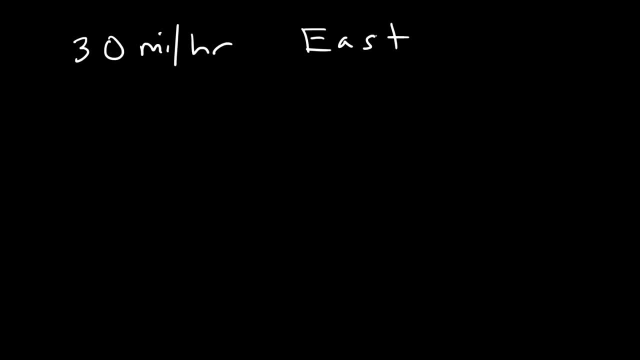 So speed tells you how fast the distance is changing. Velocity tells you how fast the displacement is changing. So let's say if a car or let's say if an object is moving at a speed of 8 meters per second, Every second the distance is changing by 8 meters. 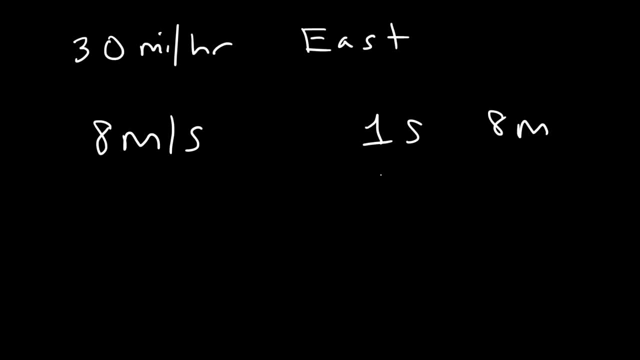 So after 1 second the distance traveled is 8 meters. 2 seconds: 60 meters. 3 seconds, 24 meters. So that's the main concept between speed and velocity. It tells you how fast the distance or the displacement is changing. 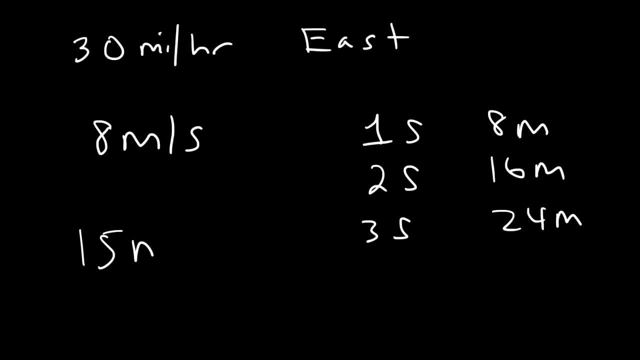 Every second. So if a car is moving at a speed of 15 meters per second, Every second the distance is changing by 15 meters. So to sum up what we just considered: Speed tells you how fast the distance is changing. 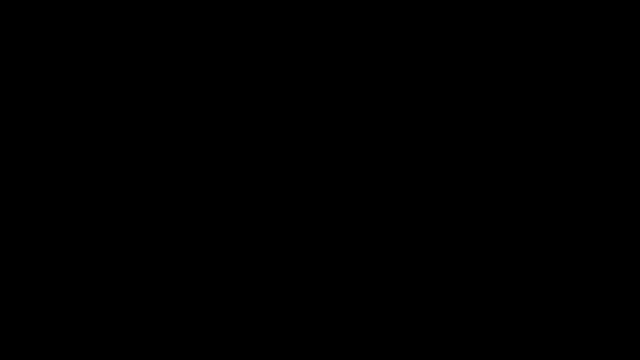 speed tells you how fast the distance is changing. Velocity tells you how fast the displacement is changing. Acceleration tells you how fast the velocity is changing. So acceleration, this is average acceleration. it's equal to the change in velocity. you can say delta v if you want to. 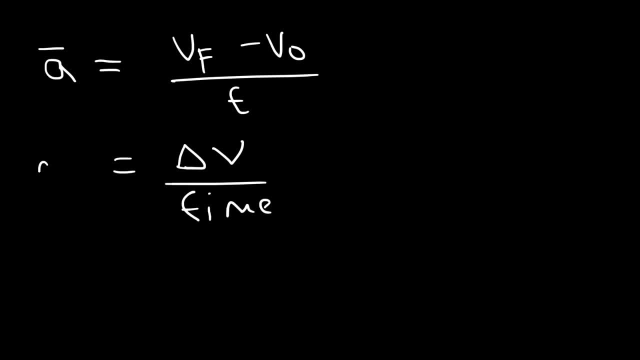 over time, That'll give you the average acceleration. If you want to find the instantaneous acceleration, as t approaches 0, when t becomes very small- that is the change in time- this expression will give you the instantaneous acceleration, But if it's over a significant time interval, 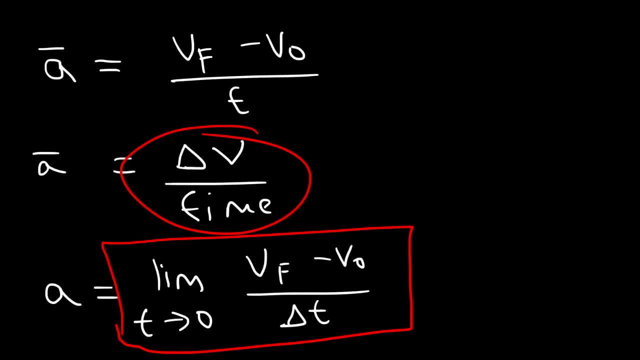 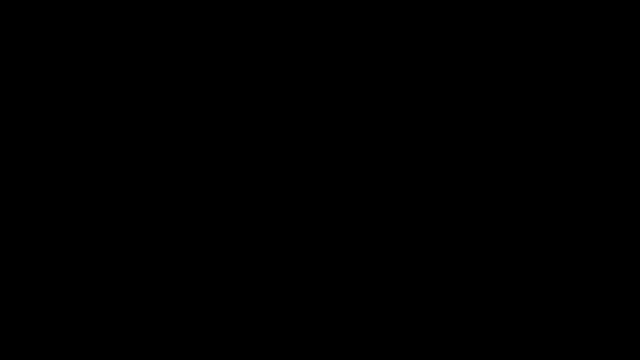 then that equation will give you the average acceleration. So just as speed tells you how fast the distance is changing, acceleration tells you how fast the velocity is changing. So let's say, if the acceleration is 8 meters per second, squared, So that means every second the velocity is changing. 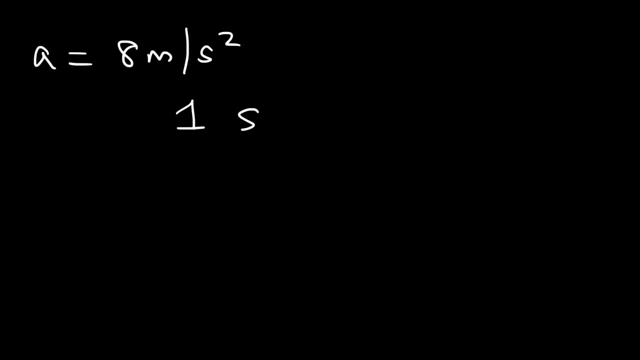 by 8 meters per second. So in one second let's say, let's make a table, Let's say: this is time and velocity. After one second the speed will be 8 meters per second. After two seconds, the velocity will be 16.. 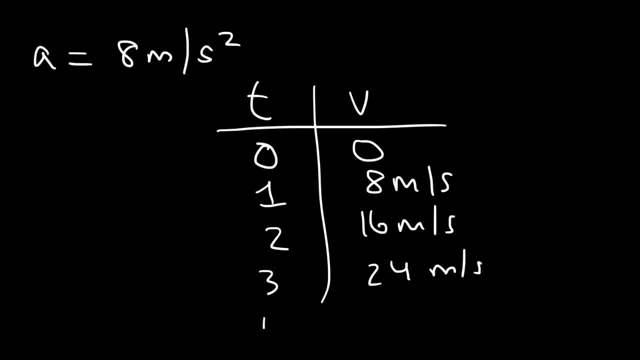 Three seconds 24.. And then four seconds 32.. So every second the velocity is increasing by 8.. So that's the main idea behind acceleration: It tells you how fast the velocity is changing. Now, starting from this equation, 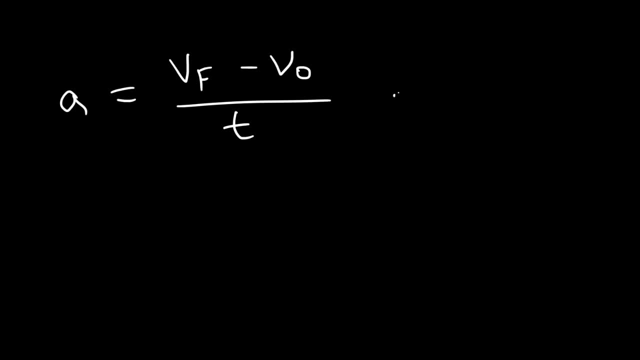 there's another equation that you might find useful. Let's multiply both sides by t, So at is equal to v final minus v initial. Now let's add v initial to both sides, So v initial plus at is equal to v final. 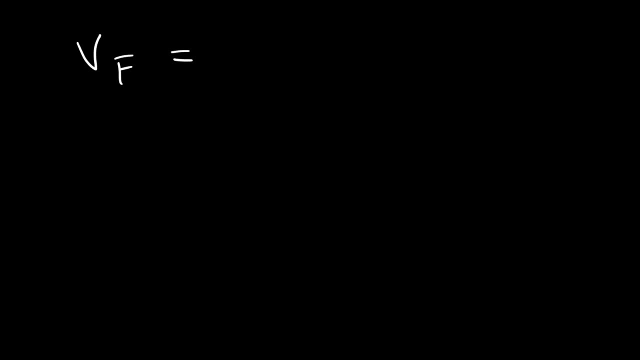 So any time you want to calculate the final speed for a motion or any object that's undergoing accelerated motion, you can use this equation. The acceleration has to be constant, by the way, for this to work. So when an object is moving with constant acceleration, 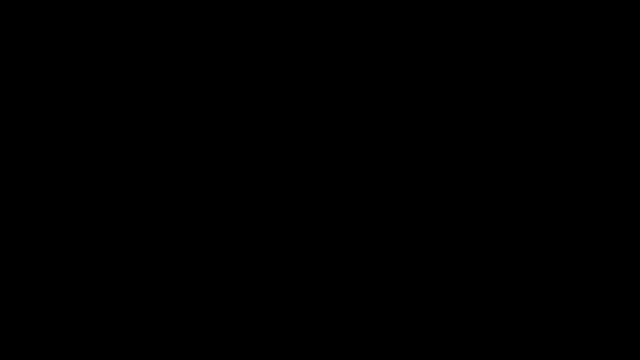 Velocity tells you how fast the displacement is changing. Acceleration tells you how fast the velocity is changing. So acceleration, this is average acceleration, it's equal to the change in velocity. you can say delta v if you want to over time. 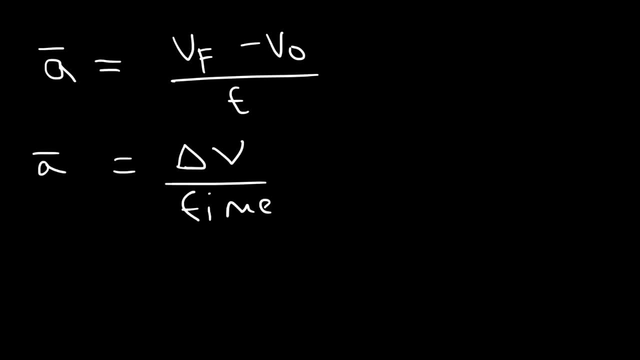 That'll give you the average acceleration. If you want to find the instantaneous acceleration as t approaches 0, when t becomes very small- that is the change in time- this expression will give you the instantaneous acceleration. But if it's over a significant time interval, then that equation will give you the average acceleration. 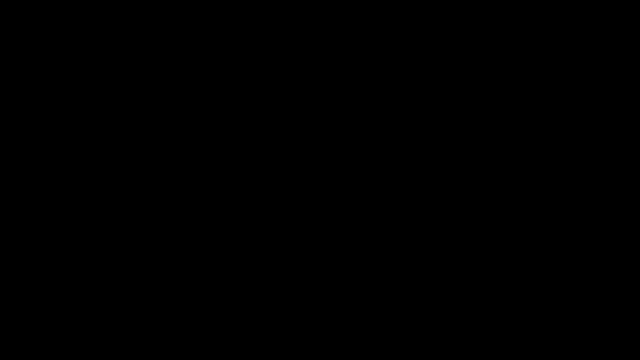 So just as speed tells you how fast the distance is changing, acceleration tells you how fast the velocity is changing. So let's say, if the acceleration is 8 meters per second, squared, So that means every second the velocity is changing by 8 meters per second. 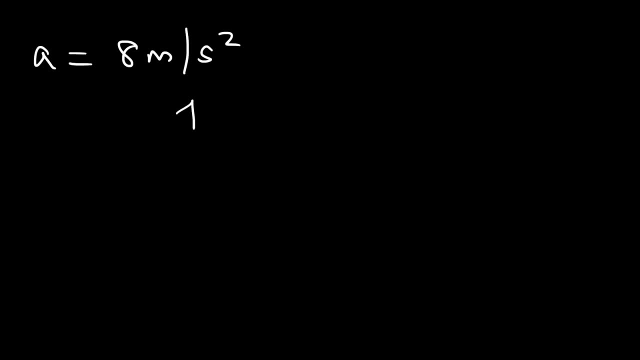 So in one second, let's say: Let's make a table, Let's say: this is time and velocity. After one second the speed will be 8 meters per second. After two seconds, the velocity will be 16.. Three seconds: 24.. 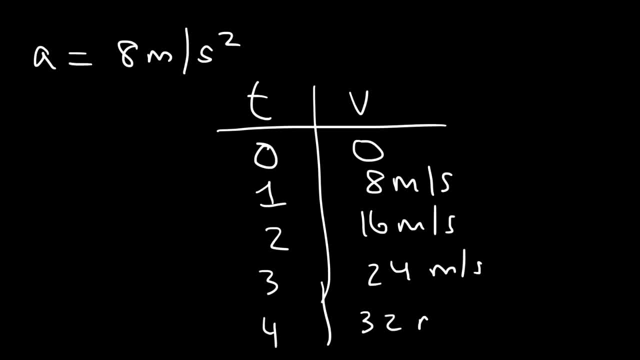 And then four seconds, 32.. So every second the velocity is increasing by 8.. So that's the main idea behind acceleration: It tells you how fast the velocity is changing. Now, starting from this equation, there's another equation that you might find useful. 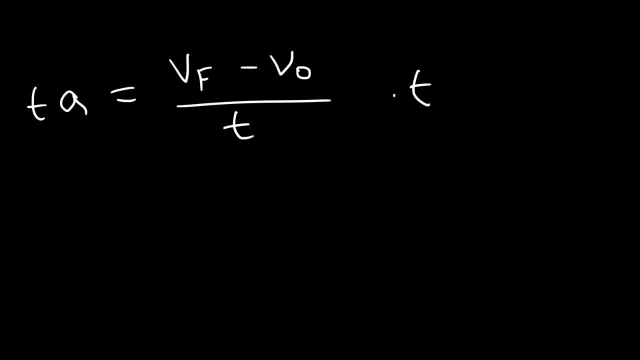 Let's multiply both sides by t, So a t is equal to v final minus v initial. Now let's add v initial to both sides, So v initial plus a t is equal to v final. So any time you want to calculate the final speed, 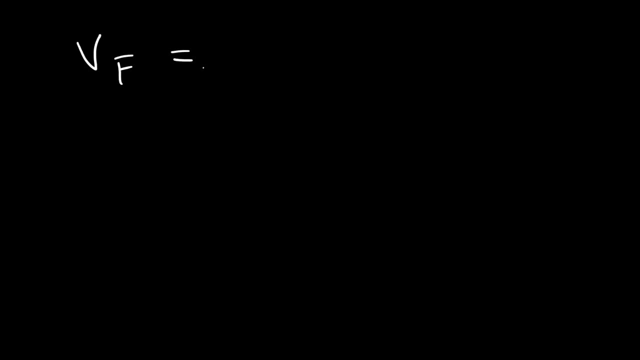 Any object that's undergone accelerated motion, you can use this equation. The acceleration has to be constant, by the way, for this to work. So when an object is moving with constant acceleration, you can find the final speed given the initial speed, the acceleration and the time. 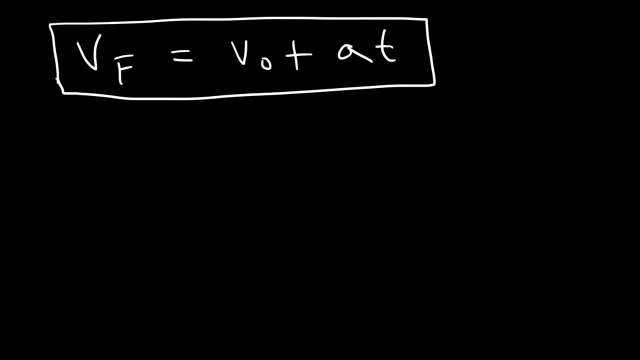 you could find the final speed given the initial speed, the acceleration and the time. Now let's work on some problems. A car accelerates from 15 meters per second to 45 meters per second in 5 seconds. Calculate the average acceleration of the car. 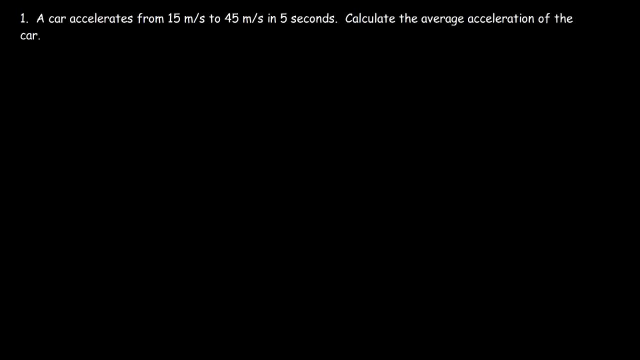 Now what I like to do is I like to make a list of what I have and what I need to find. So the initial speed in this problem is 15 meters per second. The car accelerates from that speed to a final speed. 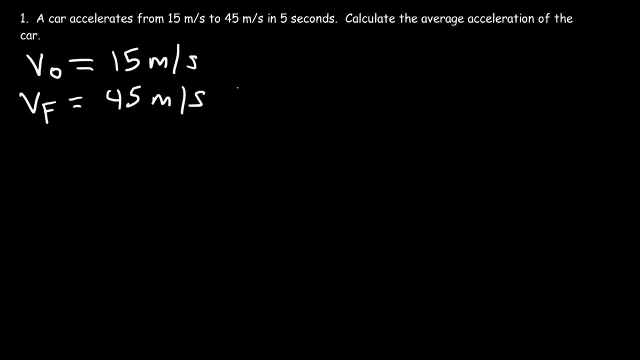 of 45 meters per second. The time in between those two points is 5 seconds. Our goal is to calculate the average acceleration, So the formula that we could use is this one. Acceleration is equal to v final minus v initial, divided by t. 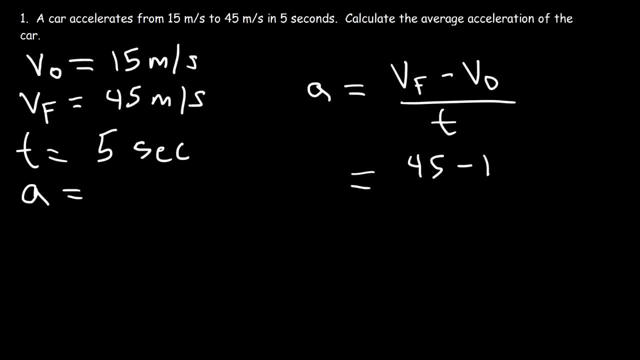 The final speed is 45. The initial speed is 15. And the time is 5.. So the change in speed is 30 meters per second And we're going to divide that by 5 seconds. 30 divided by 5 is 6.. 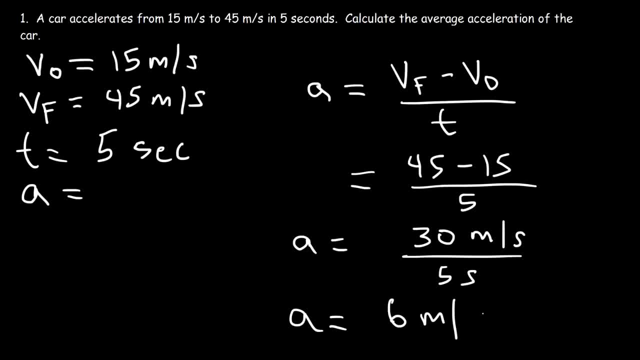 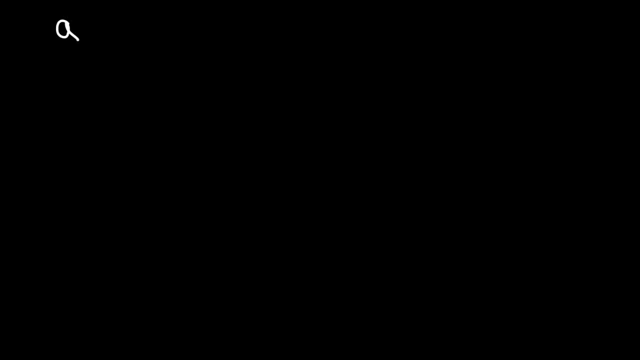 So the acceleration is 6 meters per second, squared. Now let's understand this problem. So let's make a table. So this is the acceleration. Let's make a table between time and velocity At t equals 0, the initial speed. 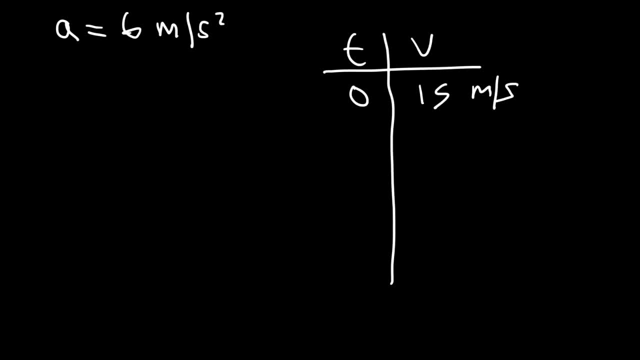 is 15 meters per second. Now keep in mind the acceleration tells us how much the speed changes, or the velocity changes, every second. So one second later it's going to be 6 meters per second higher. So 15 plus 6 is 21.. 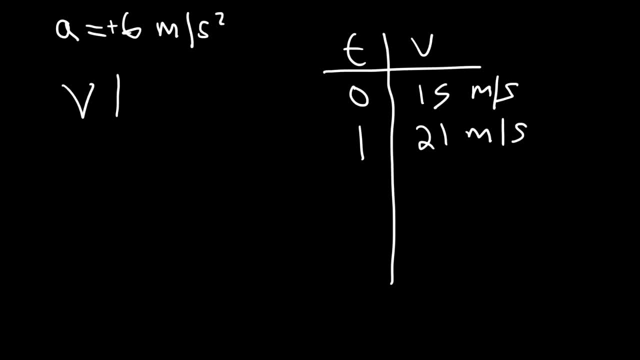 Whenever the acceleration is positive, the velocity is increasing. Two seconds later it's going to be at 27.. So every second the speed is going to increase by 6 meters per second. So at 3 seconds it's going to be 33.. 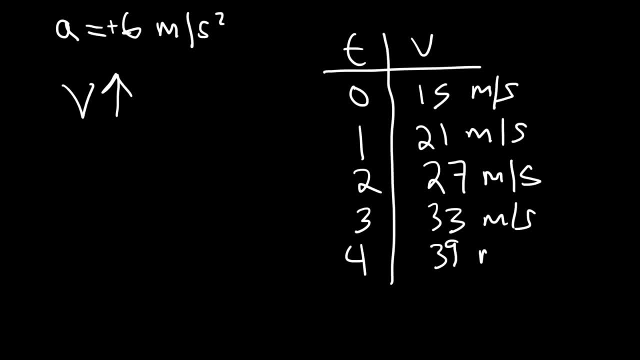 And at 4 seconds it's going to be 39.. And 5 seconds later it's going to reach to our final speed of 45 meters per second. So I want you to understand the concept of acceleration And just think of it as. 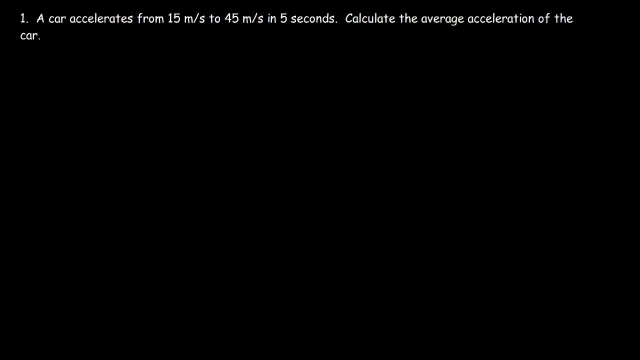 Now let's work on some problems. A car accelerates from 15 meters per second to 45 meters per second in 5 seconds. Calculate the average acceleration. What can I do to calculate the total acceleration of the car? Now, what I like to do is I like to make a list of what I have and what I need to find. 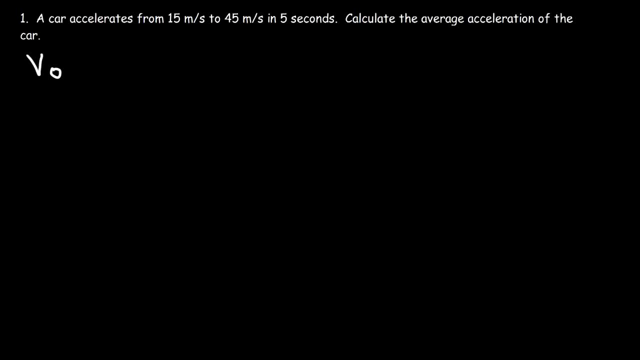 So the initial speed in this problem is 15 meters per second. The car accelerates from that speed to a final speed of 45 meters per second. The time in between those two points is 5 seconds. Calculate the acceleration. Calculate the acceleration. 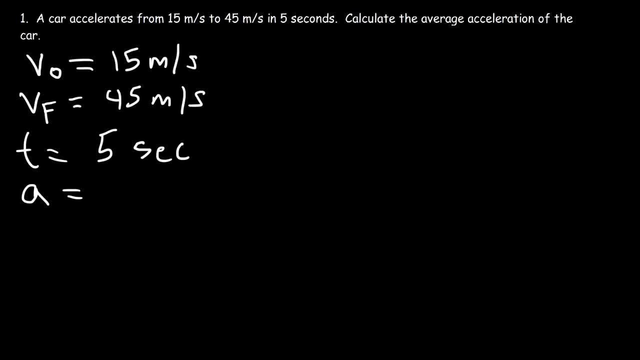 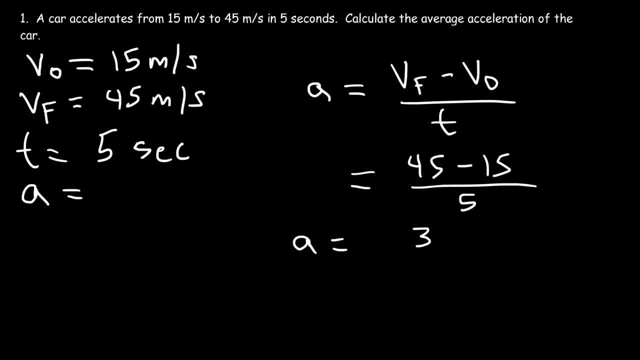 So the change in speed is 30 meters per second and we're going to divide that by 5 seconds. 30 divided by 5 is 6.. So the acceleration is 6 meters per second squared. Now let's understand this problem. 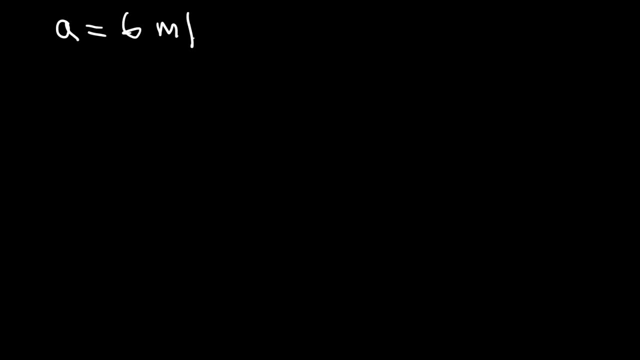 So let's make a table. So this is the acceleration. Let's make a table between time and velocity. At t equals 0,, the initial speed is 15 meters per second. Now keep in mind: the acceleration tells us how much the speed changes, or the velocity. 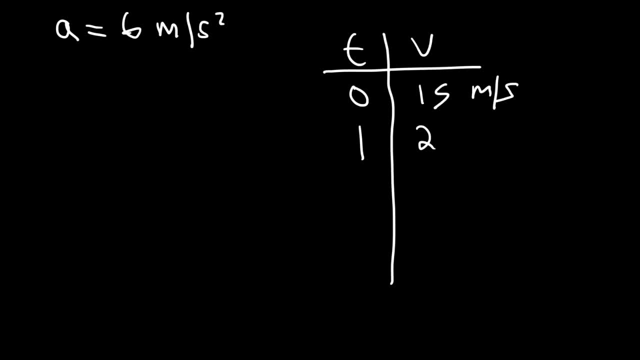 changes every second. So one second later it's going to be 6 meters per second higher. So 15 plus 6 is 21.. Whenever the acceleration is positive, the velocity is increasing. Two seconds later, it's going to be at 27.. 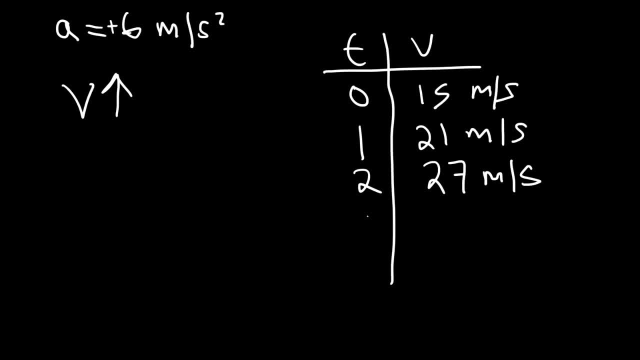 So every second the speed is going to increase by 6 meters per second. So at 3 seconds it's going to be 33.. And at 4 seconds it's going to be 39. And 5 seconds later it's going to reach to our final speed of 45 meters per second. 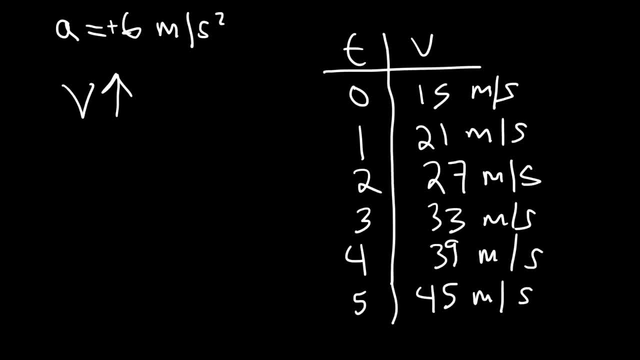 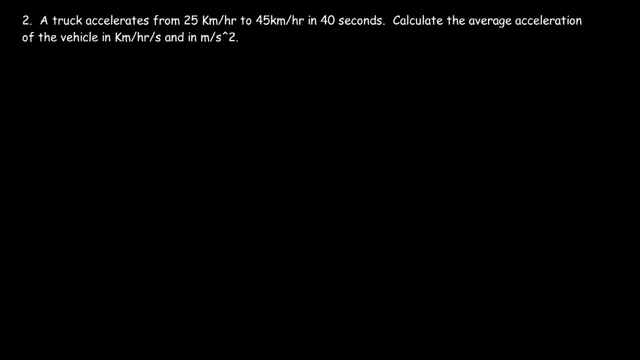 So I want you to understand the concept of acceleration And just think of it as how fast the speed changes or how fast the velocity changes every second. Number two: a truck accelerates from 25 kilometers per hour to 45 kilometers per hour in 40 seconds. 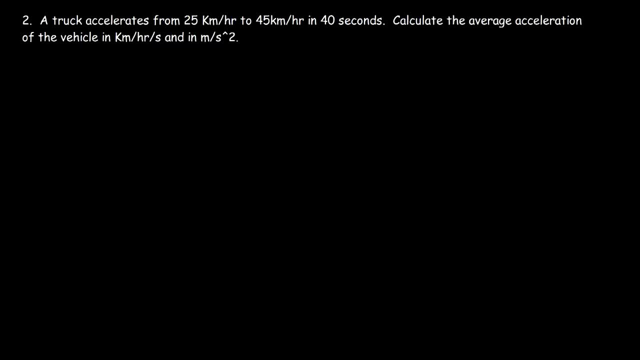 Calculate the average acceleration of the vehicle In kilometers per hour per second and in meters per second squared. So go ahead and take a minute and work on this problem. So, just like before, we're going to make a list of what we have and what we need to find. 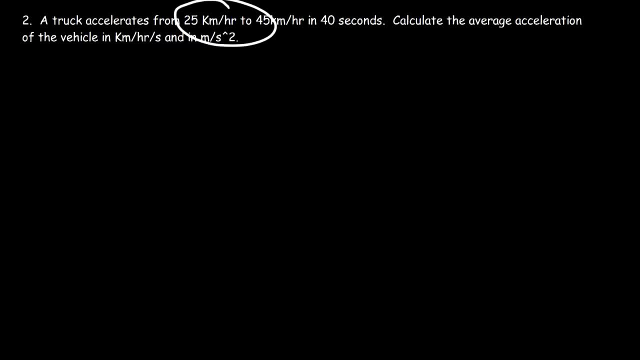 So what does the 25 kilometer per hour value represent? So that is the initial speed of the vehicle. Now we know that the final speed has to be 45 kilometers per hour, And the time in between these two events is 40 seconds. 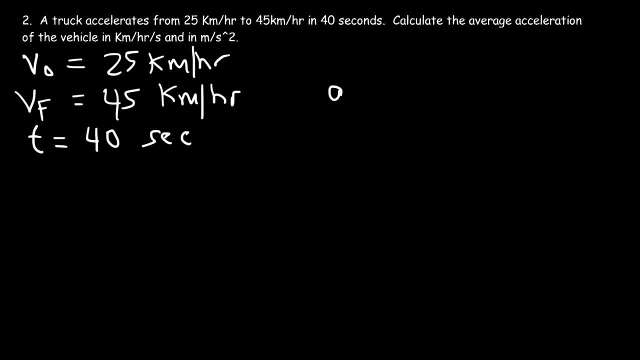 So now we could use the same formula to calculate the average acceleration. So the average acceleration is the change in the velocity divided by the time. The final speed is 45,, the initial speed is 25, and the time is 40. So 45 minus 25.. 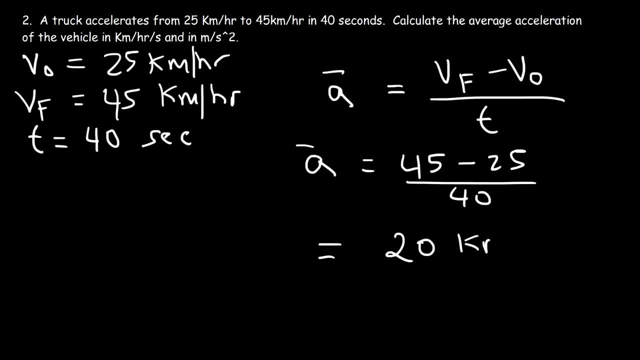 That gives us a change of 20.. And the units is kilometers per hour. And let's divide that by 40 seconds. Well, 20 divided by 40 is the same as 2 divided by 4, which is 1 half or 0.5. 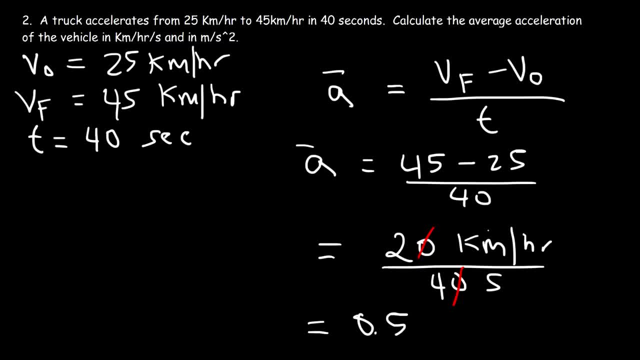 Now notice what the units for this acceleration will be. We have kilometers hours divided by seconds, So the units is going to be kilometers per hour, 1.5. Per second. So that's our answer. That's the acceleration. Now let's focus on the second part of the problem. 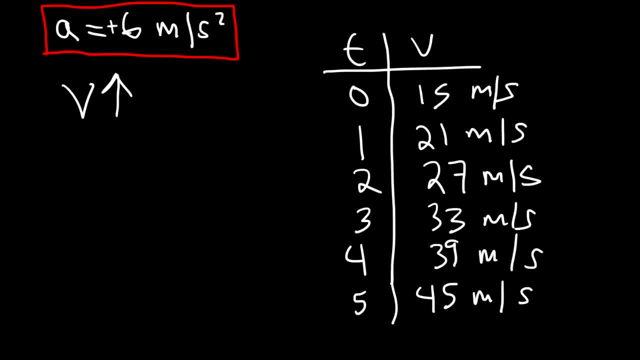 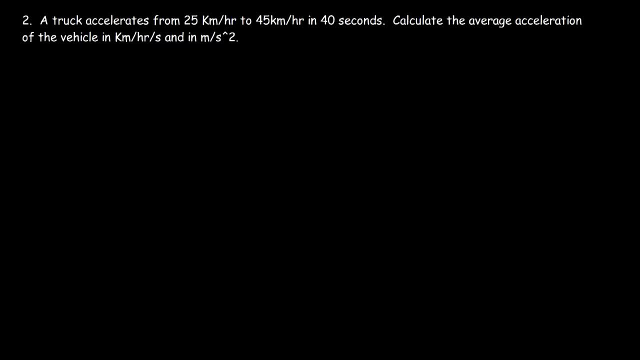 how fast the speed changes or how fast the velocity changes every second Number. 2. A truck accelerates from 25 kilometers per hour to 45 kilometers per hour in 40 seconds. Calculate the average acceleration of the vehicle in kilometers per hour per second. 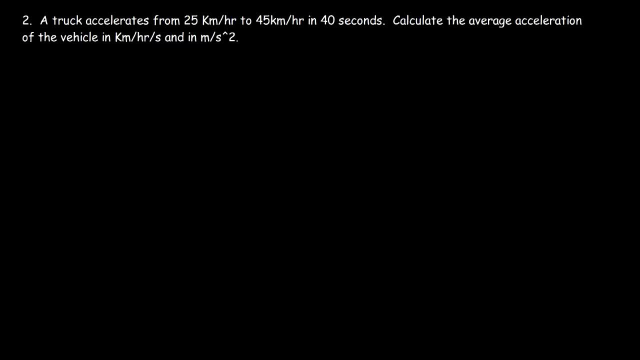 and in meters per second squared. So go ahead and take a minute and we're going to swap. So, just like before, we're going to make a list of what we have and what we need to find. So what does the 25 kilometers per hour? 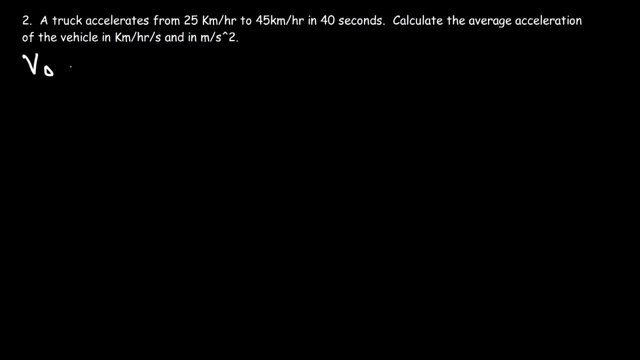 value represent. So that is the initial speed of the vehicle. Now we know that the final speed has to be 45 kilometers per hour, And the time in between these two events is 40 seconds. So now we could use the same formula to calculate. 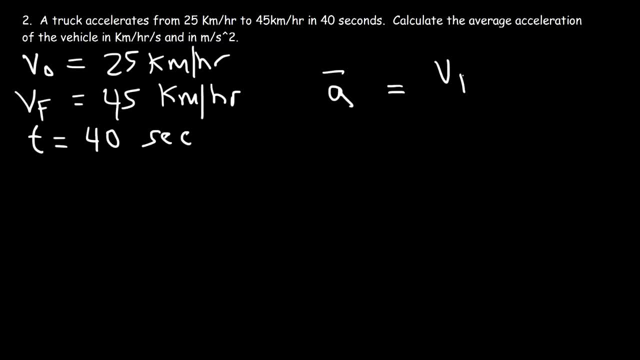 the average acceleration. So the average acceleration is the change in the velocity divided by the time. The final speed is 45., The initial speed is 25. And the time is 40. So 45 minus 25. That gives us a change. 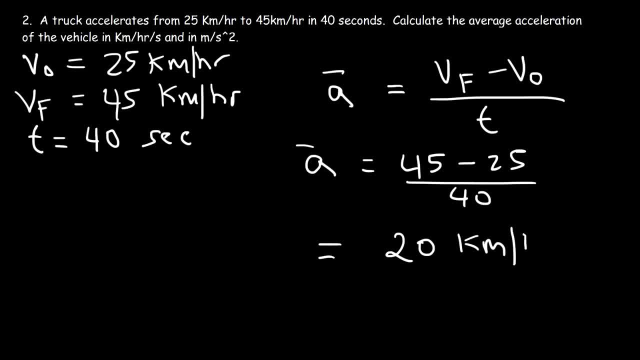 of 20. And the unit is kilometers per hour. And let's divide that by 40 seconds. Well, 20 divided by 40 is the same as 2 divided by 4, which is 1 half or 0.5.. 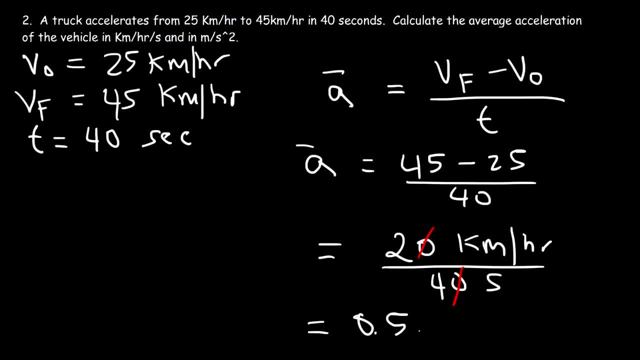 Now notice what the units for this acceleration will be. We have kilometers, hours divided by seconds, So the units is going to be kilometers per hour, per second. So that's our answer. That's the acceleration. Now let's focus on the second part. 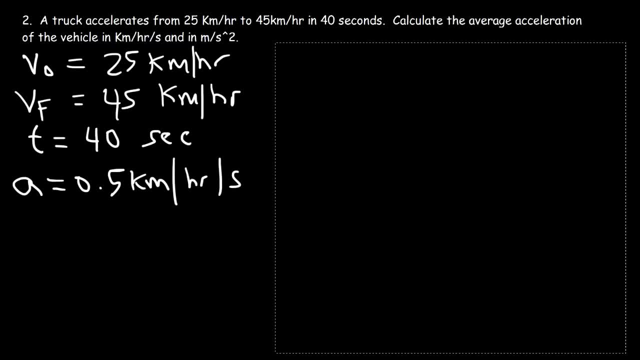 of the problem. We need to convert this unit to meters per second squared, which is the most common unit, you'll see, for acceleration. So how should we divide this? on the first fraction, 0.5 has to go on top and kilometers. 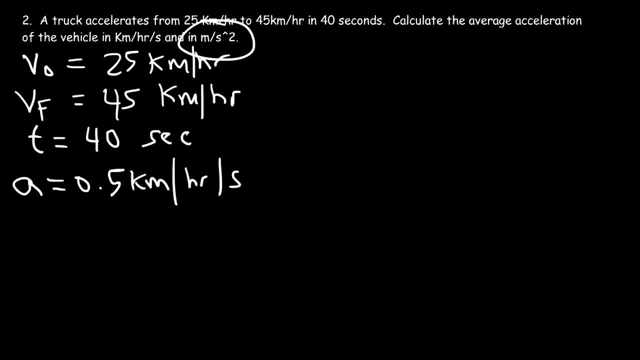 We need to convert this unit to meters per second squared, which is the most common unit you'll see for acceleration. So how should we divide this? on the first fraction, 0.5 has to go on top, and kilometers, It's 0.5 kilometers per hour per second. 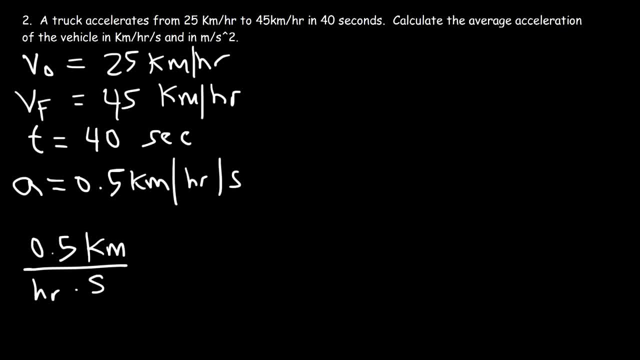 So the second two units have to go in the bottom. Now what we need to do is change kilometers to meters. One kilometer is equivalent to 1,000 meters, and we need to write it in such a way so that the unit kilometers will cancel. 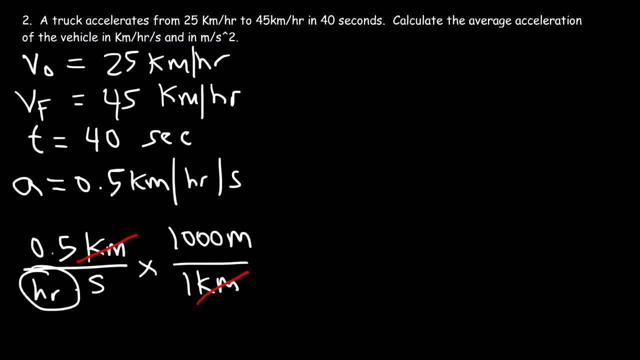 Now all we need to do is convert this hour into seconds. So one hour is equal to 60 minutes and one minute is equivalent to 60 seconds. So the unit hours cancel and the unit minutes cancel. So now we have meters per second, per second. 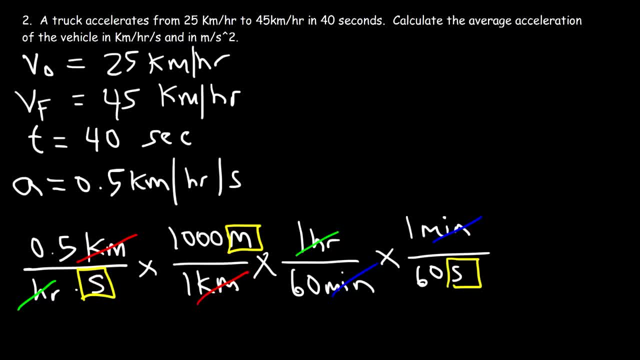 Or meters per second- per second, So that's our answer- Or meters per second squared 0.5 times 1,000 is 500.. And we're going to divide that by 60, which is about 8.33, and divide that by 60 again. 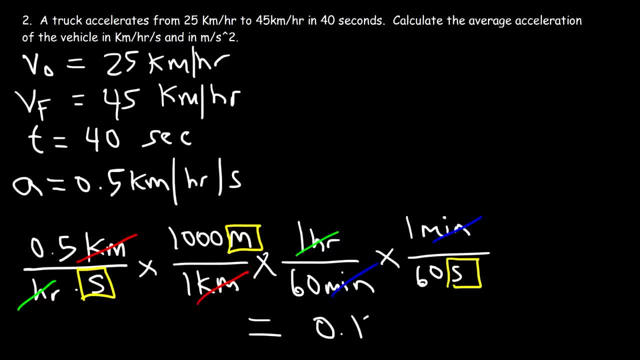 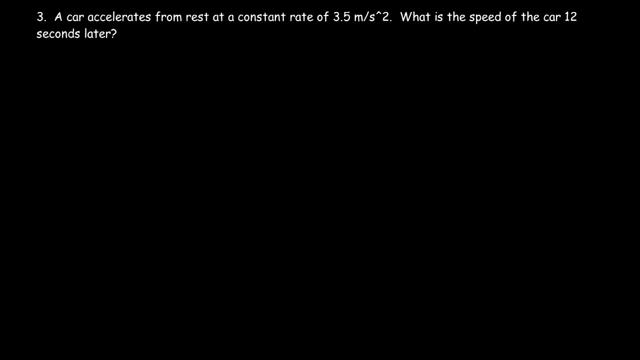 So the acceleration of this vehicle is 0.138 meters per second squared. So that's the answer. So make sure you know how to convert from one unit of acceleration into another. Here's another problem that we can work on. A car accelerates from rest at a constant rate of 3.5 meters per second squared. 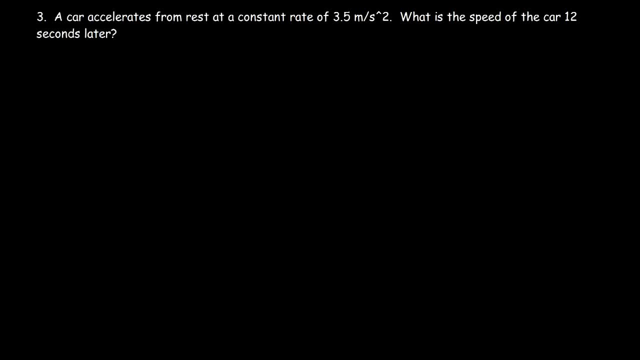 What is the speed of the car 12 seconds later? So pause the video and work on this problem. See if you can find the answer Now. what varies, What variables do we have in this problem? What is the initial speed and what is the final speed? 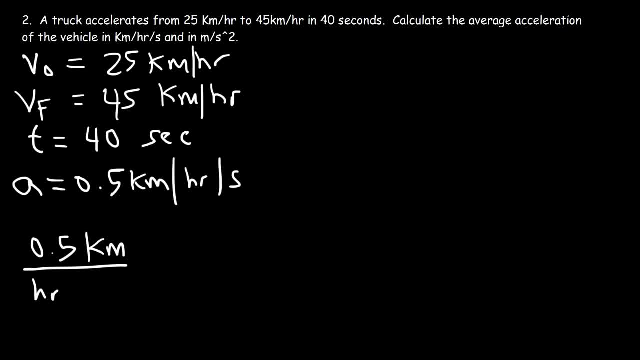 It's 0.5 kilometers per hour, per second, So the second two units have to go in the bottom. Now what we need to do is change kilometers to meters. One kilometer is equivalent to 1000 meters, And we need to write it in such a way. 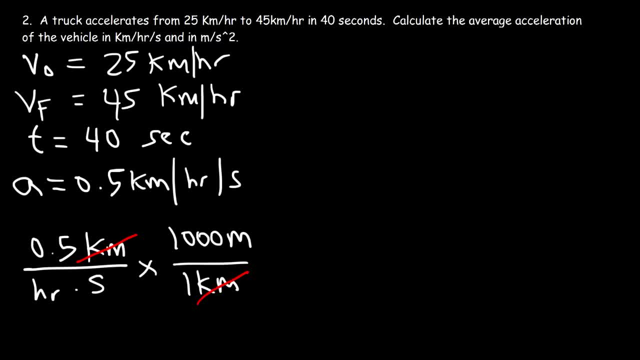 so that the unit kilometers will cancel. Now all we need to do is convert this hour into seconds. So one hour is equal to 60 minutes And one minute is equivalent to 60 seconds. So the unit hours cancel and the unit minutes cancel. 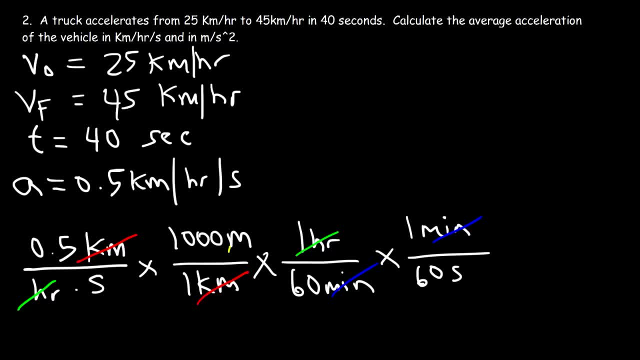 So now we have meters per second. per second, or meters per second squared 0.5 times 1000 is 500. And we're going to divide that by 60,, which is about 8.33, and divide that by 60 again. 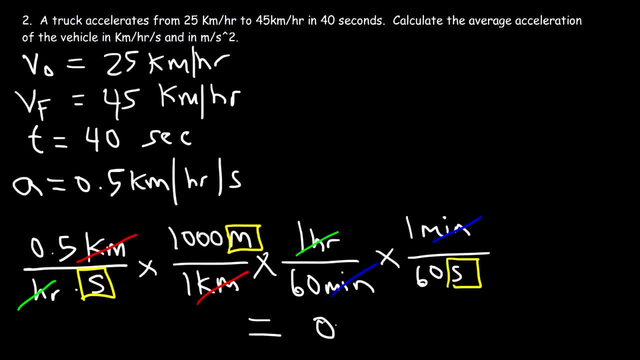 So the acceleration of this vehicle is 0.133, 8 repeating meters per second squared. So that's the answer. So make sure you know how to convert from one unit of acceleration into another. Here's another problem that we can work on. 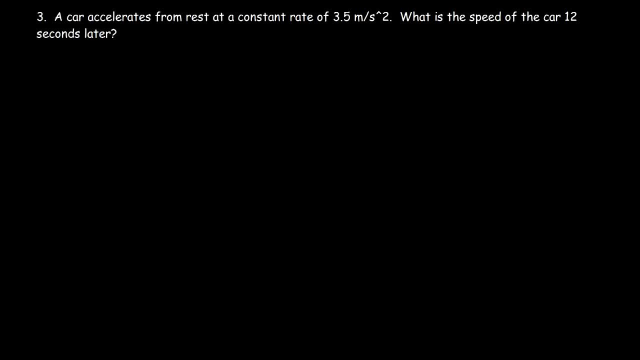 A car accelerates from rest at a constant rate of 3.5 meters per second, squared. What is the speed of the car 12 seconds later? So pause the video and work on this problem. See if you can find an answer. 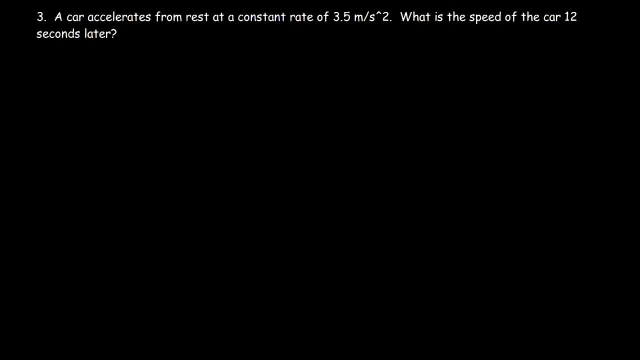 Now, what variables do we have in this problem? What is the initial speed and what is the final speed? What is the time and what is the acceleration as well? Now, whenever you hear the word rest, that tells you that the speed is 0. The car accelerates. 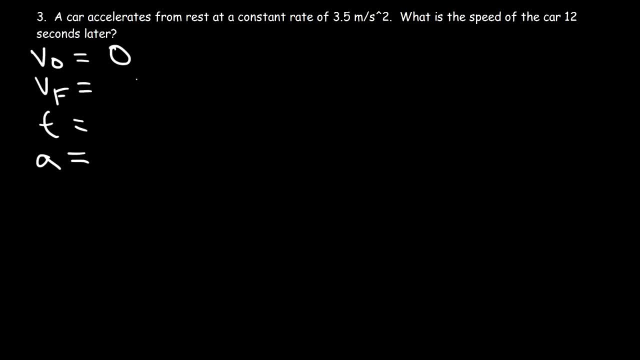 from rest. That means it's accelerating from an initial speed of 0.. Our goal is to find the final speed of the vehicle, So that's what we're looking for. The time is 12 seconds and the acceleration is 3.5 meters per. 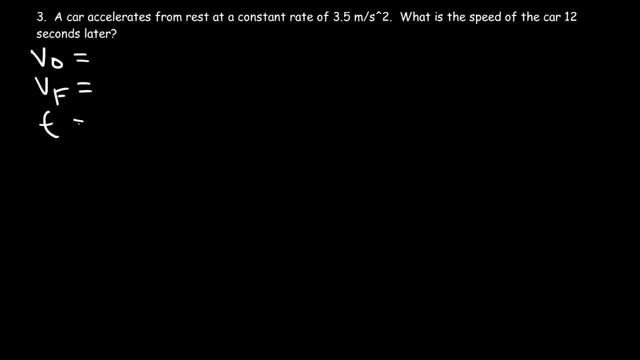 What is the time and what is the acceleration as well. Now, whenever you hear the word rest, that tells you that the speed is zero. The car accelerates from rest. That means it's accelerating from an initial speed of zero. Our goal is to find the final speed of the vehicle. 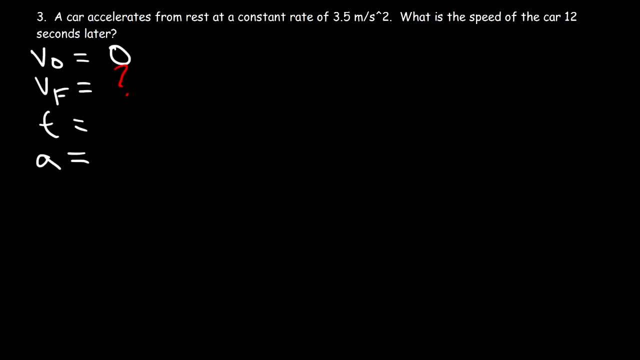 So that's what we're looking for. The time is 12 seconds and the acceleration is 3.5 meters per second squared, So what equation do we need to use in order to calculate the final speed? So we need to use this formula. 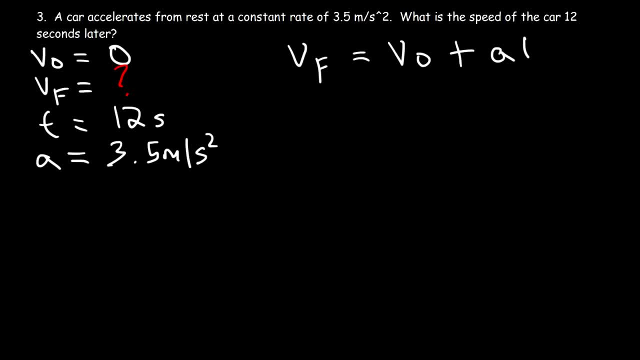 The final speed is equal to the initial speed plus the product of the acceleration and the time. The initial speed is zero, the acceleration is 3.5, and the time is 12.. So all you need to do is multiply 3.5 times 12.. 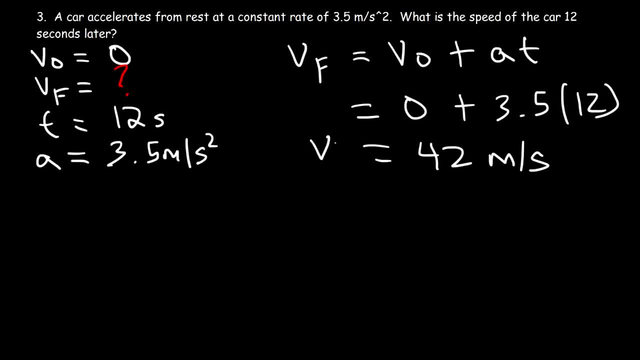 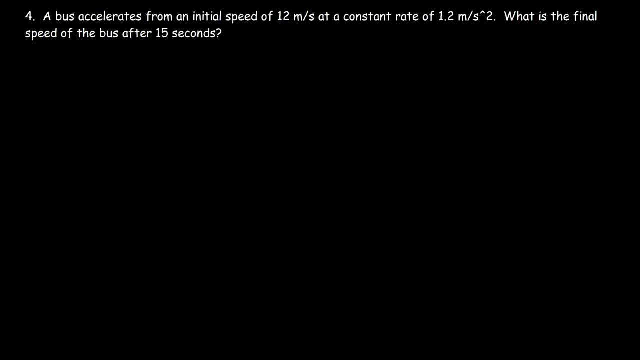 And that will give you the final speed of 42 meters per second. Number four: A bus accelerates from an initial speed of 12 meters per second at a constant rate of 1.2 meters per second. squared, What is the final speed of the bus after 15 seconds? 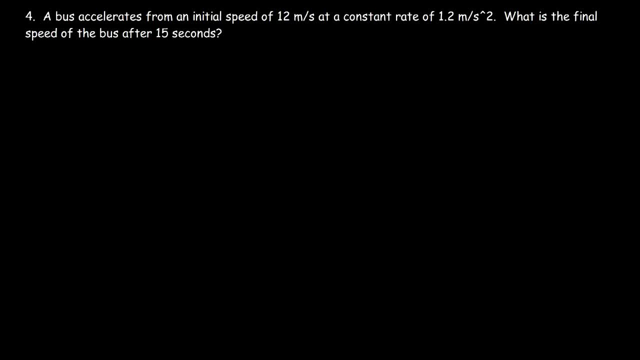 So, just like before, Let's make this a little easier. Let's make this a little easier, Let's make a list of the variables that we have and a variable that we need to find. So we're given the initial speed, which is 12 meters per second. 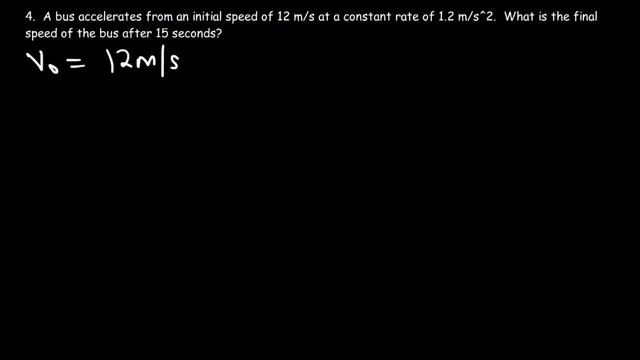 And looking at the units- meters per second squared- we can see that that value represents the acceleration And if you see the unit seconds, you know that represents time. Our goal is to find the final speed, So we need to calculate Vf. 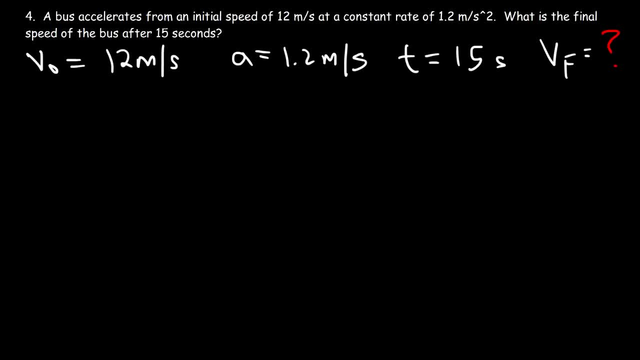 Therefore we can use the same exact equation as the one we used in the last problem. So Vf is equal to V, initial plus 80.. The initial speed is 12.. The acceleration is 1.2.. And the time is 15 seconds. 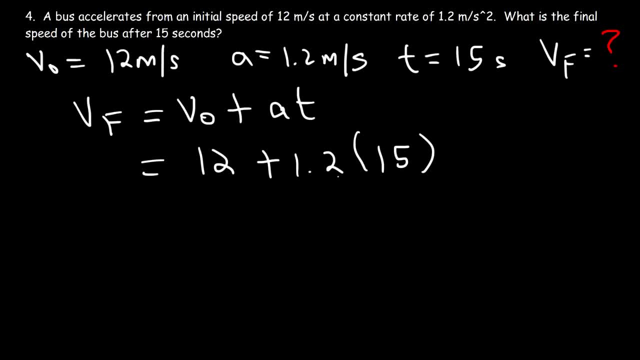 So first let's multiply 1.2 by 15.. So the initial speed is 12.. The acceleration is 1.2. And the time is 15 seconds. 1.2 times 15 is 18.. And 12 plus 18 is 30.. 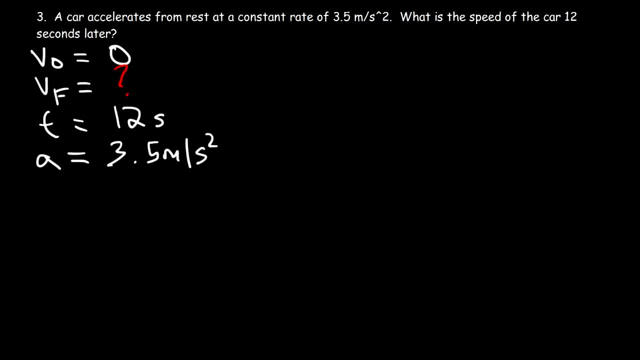 second squared. So what equation do we need to use in order to calculate the final speed? So we need to use this formula: The final speed is equal to the initial speed plus the product of the acceleration and the time. The initial speed is 0. 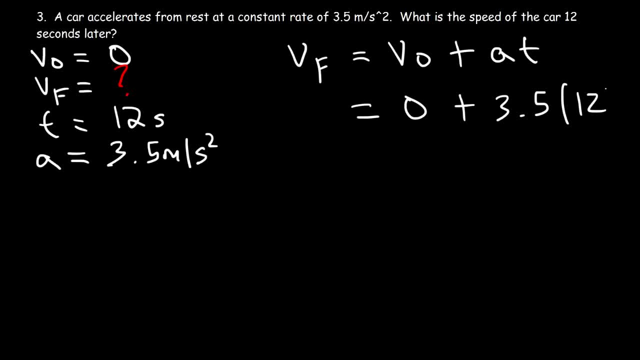 the acceleration is 3.5 and the time is 12.. So all you need to do is multiply 3.5 times 12 and that will give you the final speed of 42 meters per second. Number 4. A bus accelerates from an 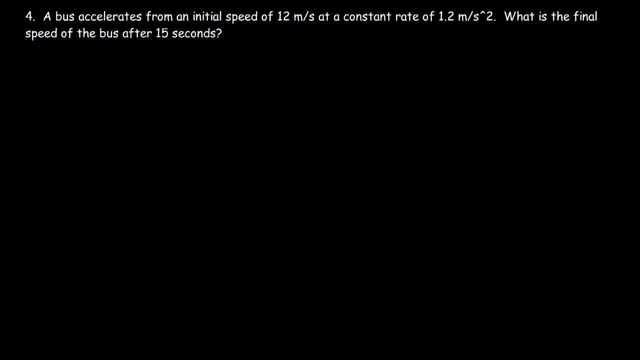 initial speed of 12 meters per second, at a constant rate of 1.2 meters per second. squared, What is the final speed of the bus after 15 seconds? So, just like before, let's make a list of the variables that we have and the 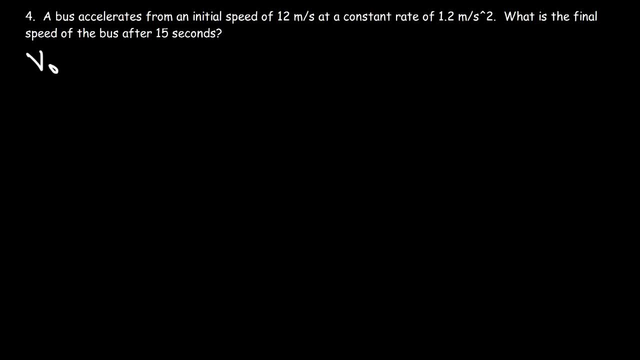 variable that we need to find. So we're given the initial speed, which is 12 meters per second, And looking at the units of meters per second squared, we can see that that value represents the acceleration. And if you see the units set, 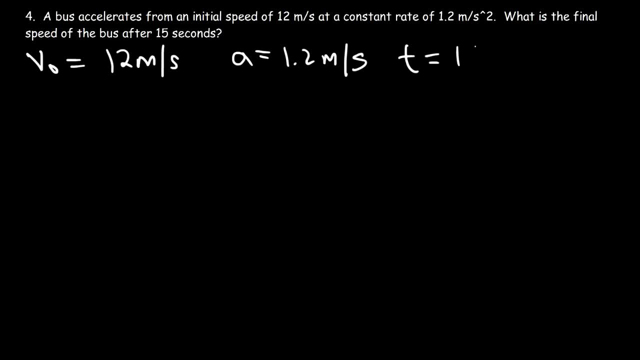 in seconds. you know that that represents time. Our goal is to find the final speed of the bus, So we need to calculate Vf. Therefore, we can use the same exact equation as the one we used in the last problem. So Vf is equal to. 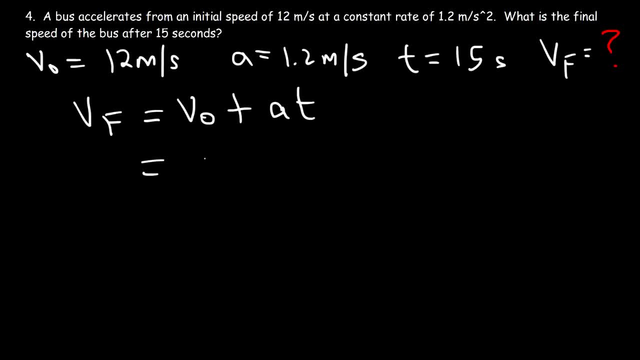 V initial plus At The initial speed is 12,, the acceleration is 1.2, and the time is 15 seconds. So first let's multiply 1.2 by 15.. 1.2 times 15 is 18.. 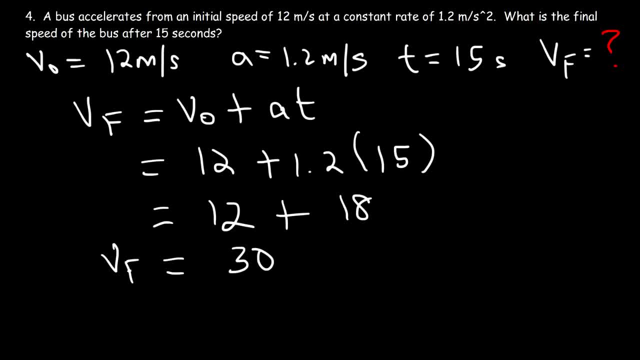 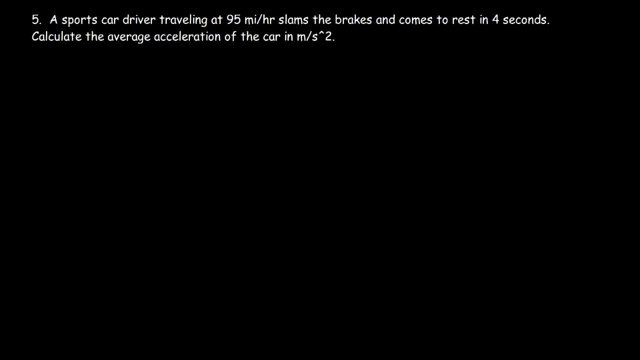 And 12 plus 18 is 30. So the final speed is 30 meters per second. Number 5. A sports car driver traveling at 95 miles per hour slams the brakes and comes to rest in 4 seconds. Calculate the average acceleration. 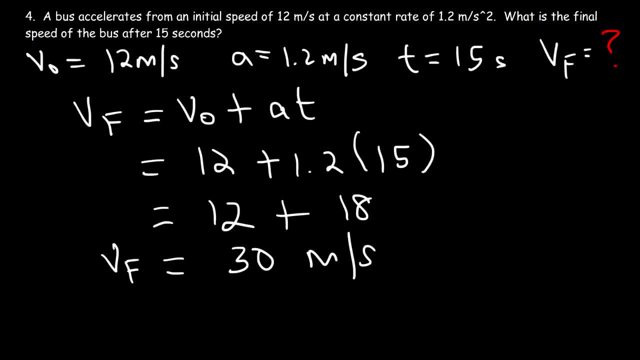 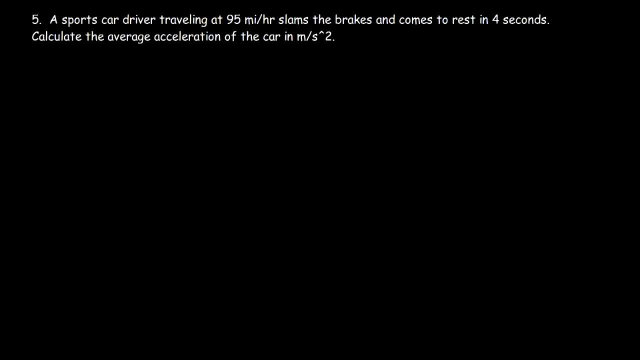 So the final speed is 30 meters per second. Number 5.: A sports car driver traveling at 95 miles per hour slams the brakes and comes to rest in 4 seconds. Calculate the average acceleration of the car in meters per second squared. 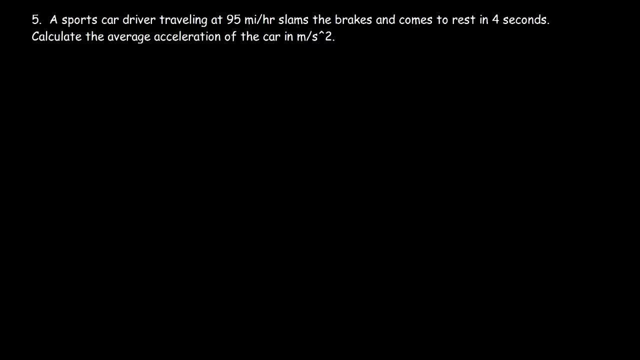 So let's think about this: If we want to find the acceleration in meters per second squared, we need to convert the speed from miles per hour to meters per second. It's not like the second problem, where we had to get the answer in terms of kilometers. 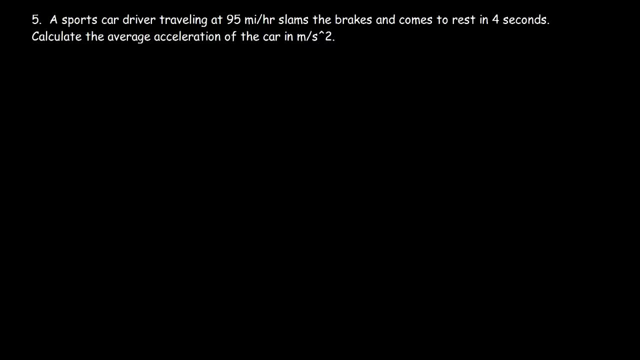 per hour per second. If we only needed to get the answer in meters per second squared, I would have changed the units from the beginning, But in this case we need to get it in meters per second squared. So let's begin by converting miles per hour to meters per second. 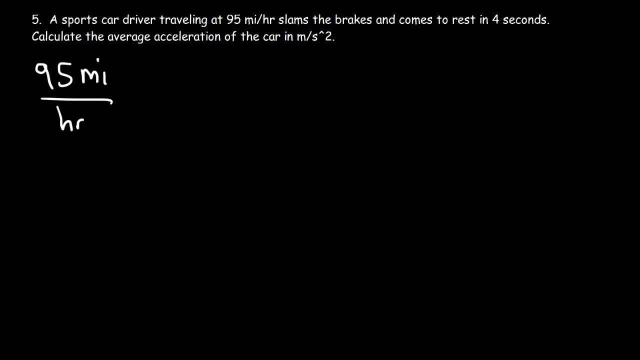 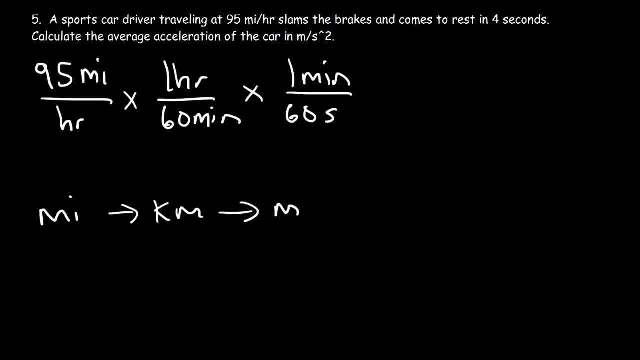 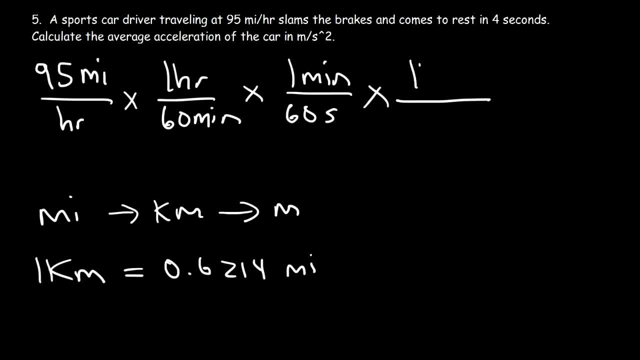 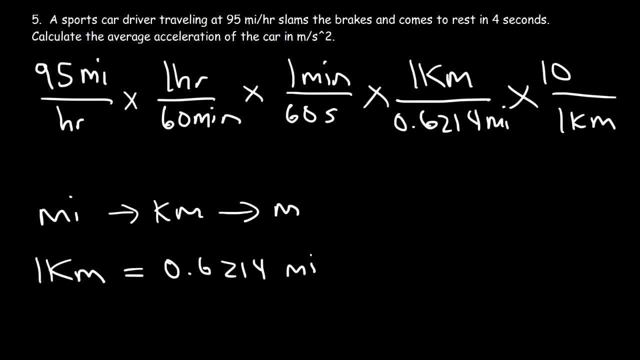 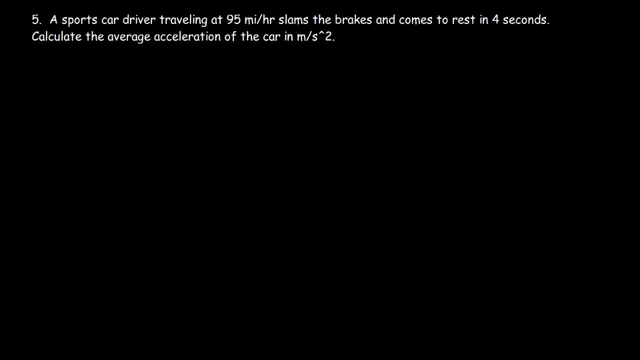 of the car in meters per second squared. So let's think about this: If we want to find the acceleration in meters per second squared, we need to convert the speed from miles per hour to meters per second. It's not like the second problem. 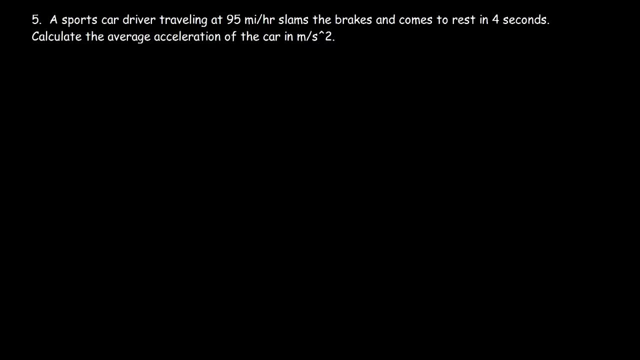 where we had to get the answer in terms of kilometers per hour per second. If we only needed to get the answer in meters per second squared, I would have changed the units from the beginning, But in this case we need to get it in meters per second squared. So 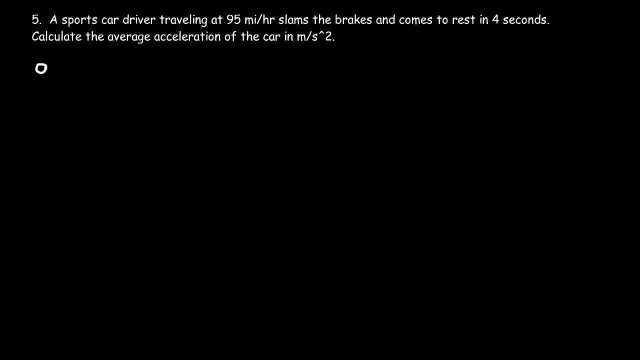 let's begin by converting miles per hour to meters per second. So we have 95 miles per hour. One hour contains 60 minutes And each minute contains 60 seconds. Now how can we convert miles to meters? One way we can do it is: 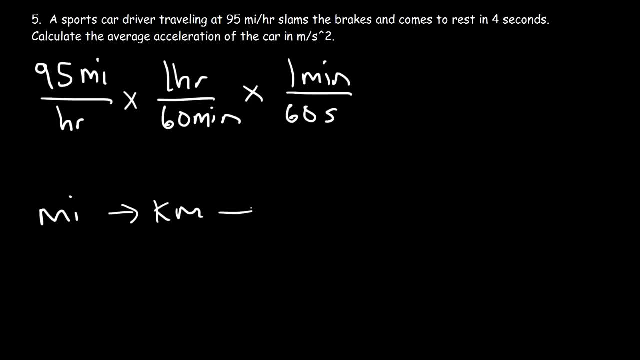 we can convert miles to kilometers and then kilometers to meters, So we need to know the conversion. If I recall, one kilometer is .6214 miles And we know that one kilometer is also 1000 meters. So, as you can see, the unit miles. 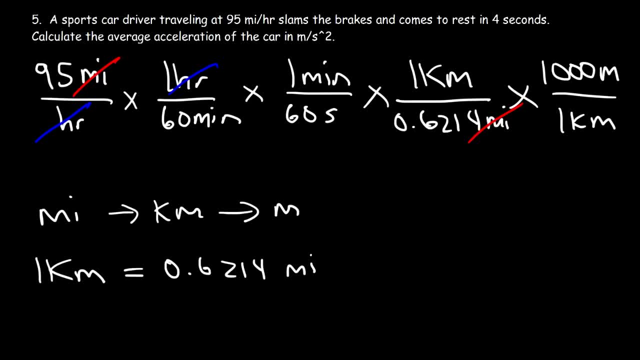 cancels Hours cancels as well. The same is true for minutes And finally kilometers. So we're left with meters per second. Now let's do the math: 95 divided by 60 divided by another 60 divided by. 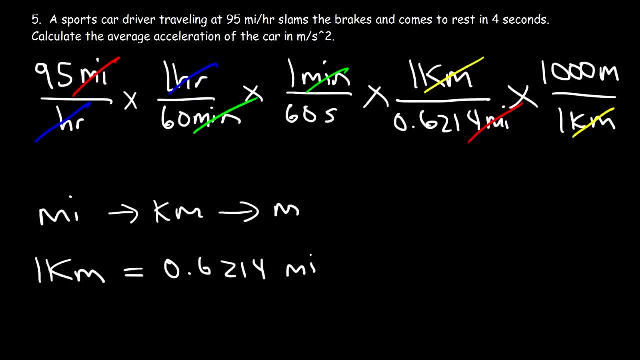 .6214 times 1000 is about 42.47.. So that's the initial speed of the vehicle. It's 42.47 meters per second. Now what is the final speed of the vehicle If the driver slams the brakes? 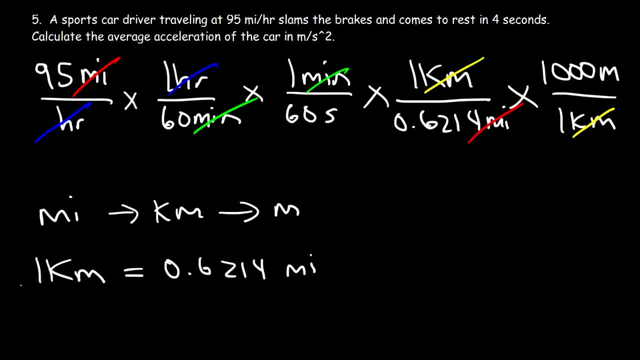 So we're left with meters per second. Now let's do the math: 95 divided by 60, divided by another 60, divided by 0.6214 times 1,000, is about 42.47.. So that's the initial speed of the vehicle. it's 42.47 meters per second. 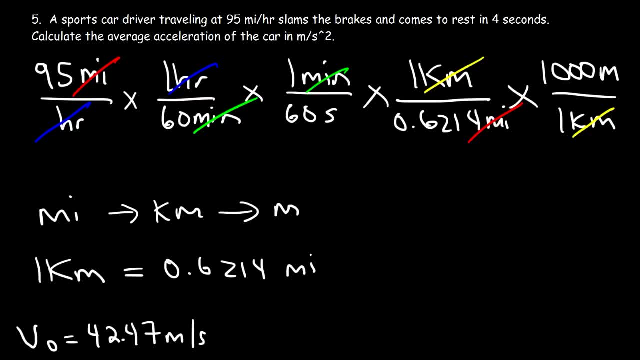 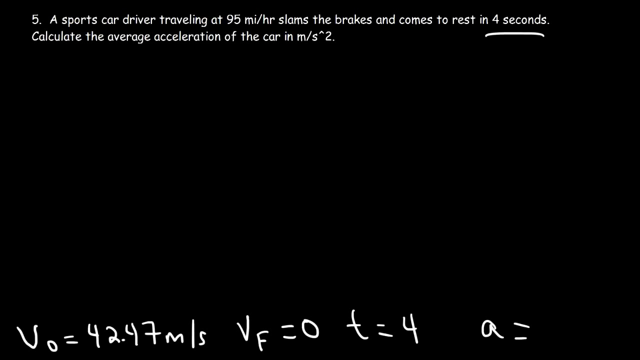 Now, what is the final speed of the vehicle? If the driver slams the brakes? he's going to come to rest eventually. So the final speed is 0.. The time we can see it's 4 seconds and our goal is to find the acceleration. 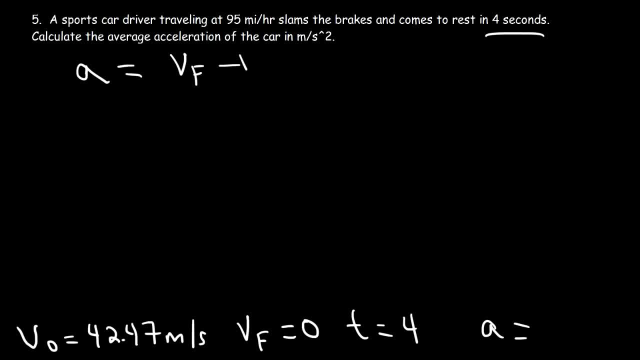 So let's use this formula. Let's use this formula: A is equal to V final minus V initial, divided by T. So it's 0 minus 42.47 divided by 4.. So negative 42.47 divided by 4, that's about negative 10.6 meters per second squared. 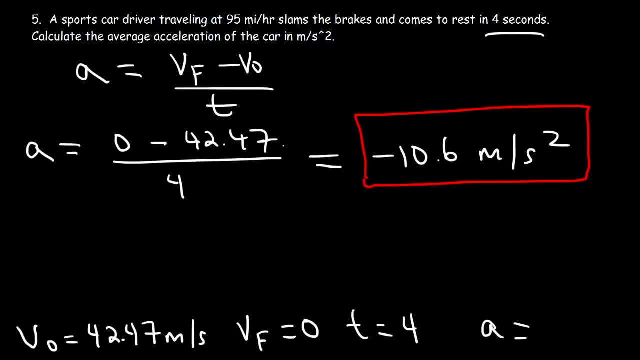 Now why is the acceleration negative? The speed is decreasing Any time the velocity is decreasing, which is the magnitude of speed. speed is the magnitude of velocity, But any time the velocity is decreasing, the acceleration will be negative. And the car is slowing down, it's coming to a stop. 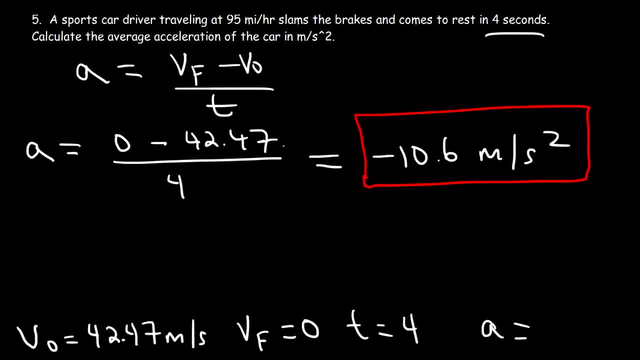 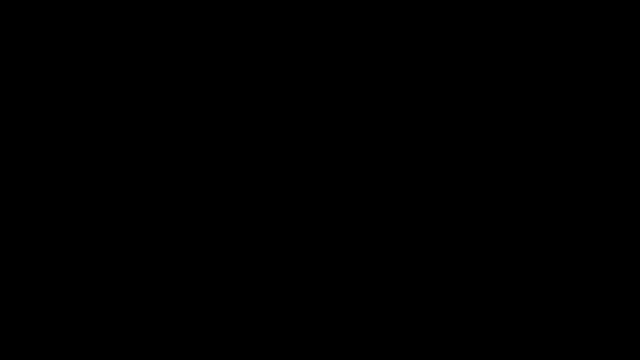 And so that's why you should have a negative average acceleration. So that's what it means When I drive.